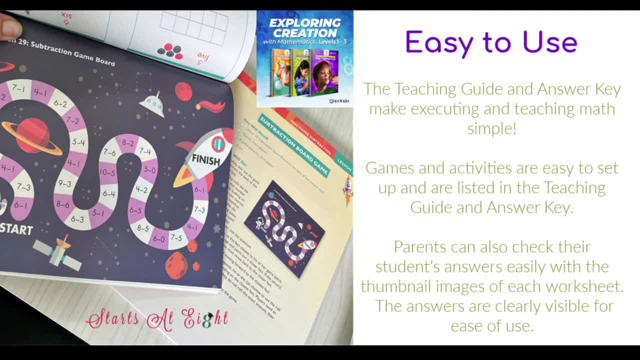 Another component that I really love about the Apologia Homeschool Elementary Math curriculum is the teacher guide and answer key. This resource makes executing and teaching math so simple. It's organized by unit. Each unit includes a full supply list, which is so great, because then at the 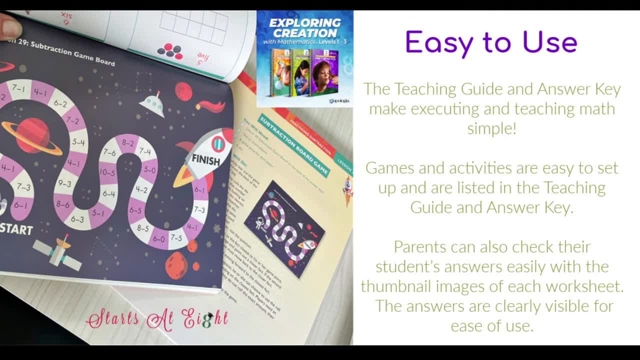 beginning of a unit, you can gather up and make sure you have all the manipulatives and things that you're going to need, so that you don't have to stop each lesson time and look for the items that you're going to be using during that lesson, As well as the full supply list. 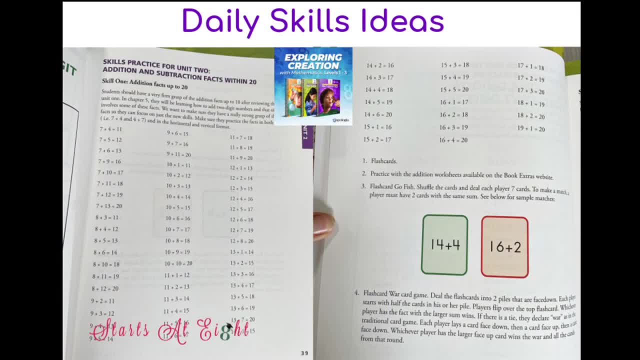 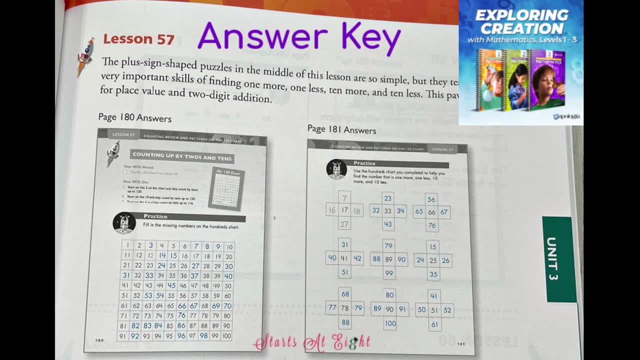 all of the daily skills ideas are found within the teacher guide, So in each unit you will find this skills practice list and ideas for how to practice those skills. Another thing you find is the answer key. What I love about this answer key, as you can see in this image, is that 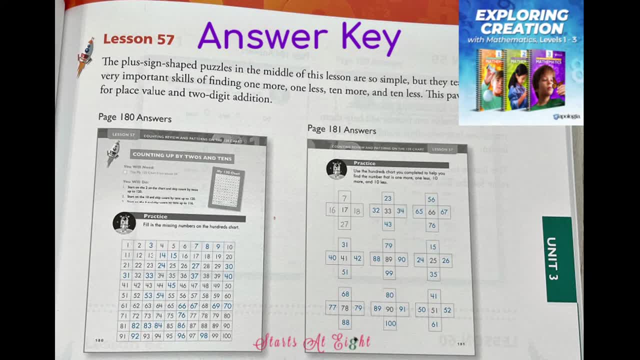 it's the answer key to the answer key. It's the answer key to the answer key. It's the answer key to the actual pages, and then it just fills in the answers in a different color. I think this makes it so much easier to grade than trying to look through a list of answers that you kind of have. 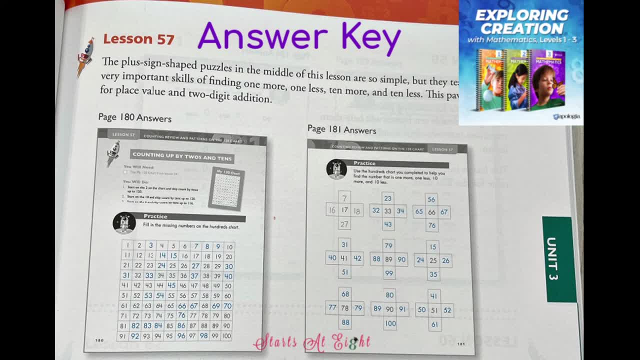 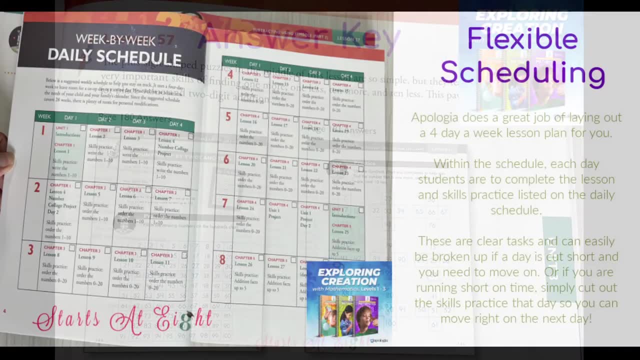 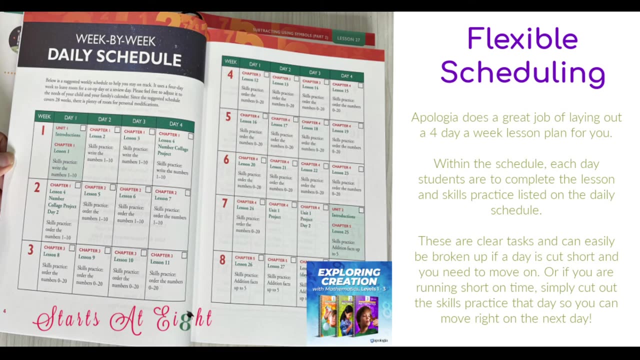 to fill in and figure out exactly where they belong. So this feature really, really makes it quick and simple to grade your kids' math. The last thing I want to talk about is the flexible scheduling. Apologia is great at this. I've seen it in their science. 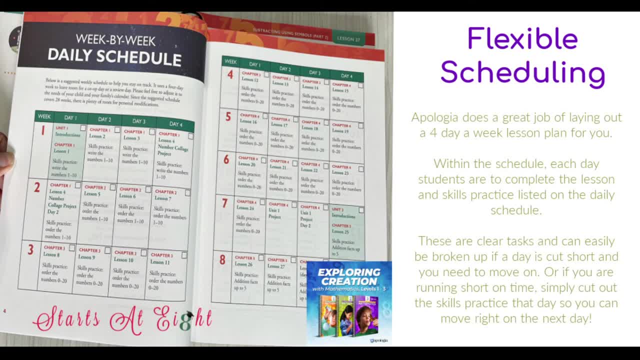 curriculum. I've seen it in their science curriculum. I've seen it in their science curriculums And now I see it here in their math curriculum. They lay out a week-by-week schedule for you, based on four days a week. That makes it so much more flexible. It builds in time for things. 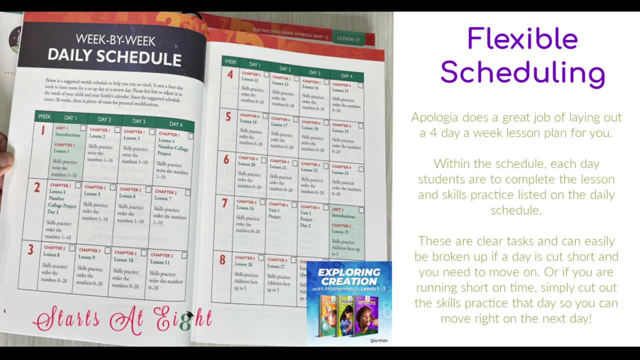 like illnesses or vacations or something just came up and you had a play date with a friend. You know there's no prep work ahead for you, There's no planning. They lay it out As you do each day. you check it off And if you say,